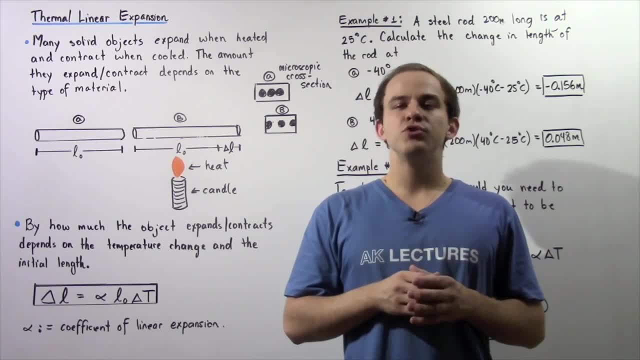 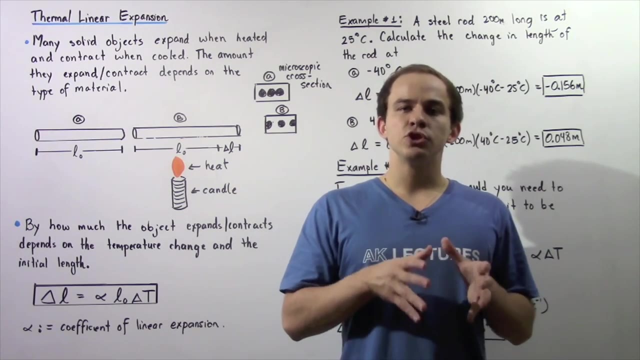 In a previous lecture we mentioned a concept known as thermal expansion of solids. So thermal expansion of solids essentially means whenever we heat or cool a solid, that object, that solid object, has the potential to expand or contract. Now there are two types of thermal expansions. 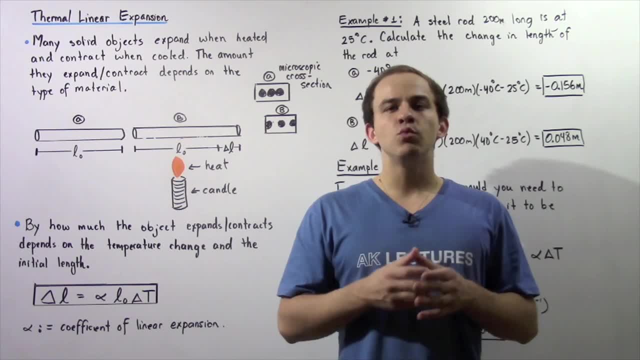 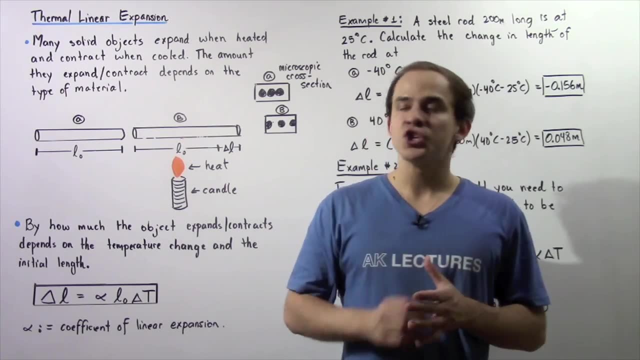 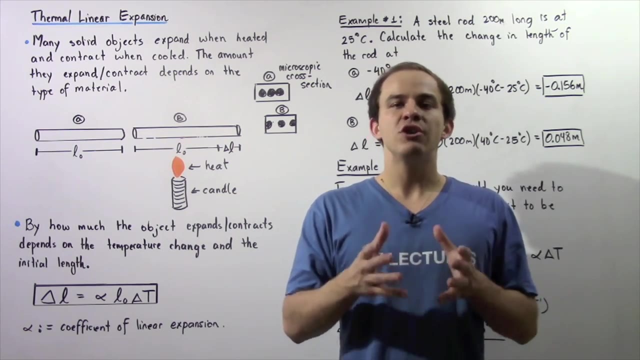 that you should know. There is volume expansion, in which the solid object expands or contracts outward in all possible directions, And there's also thermal, linear expansion, in which the solid object expands or contracts along a horizontal axis or along a vertical axis. In this lecture, 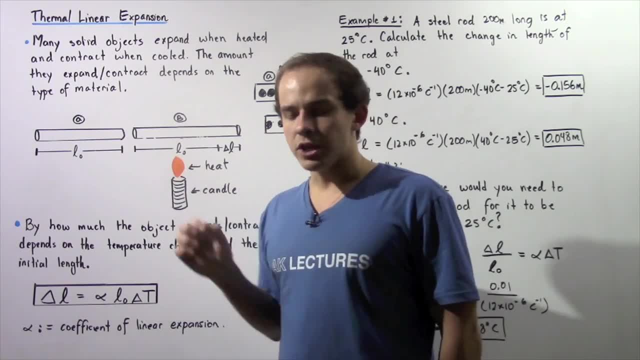 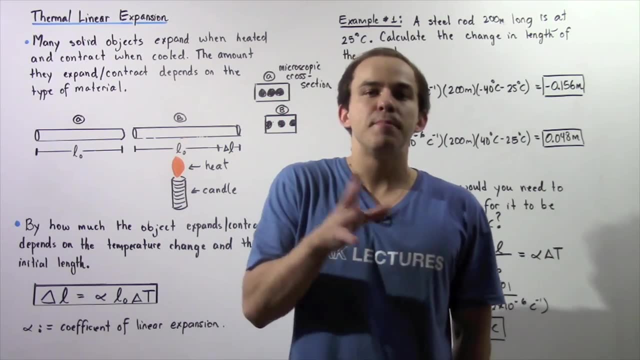 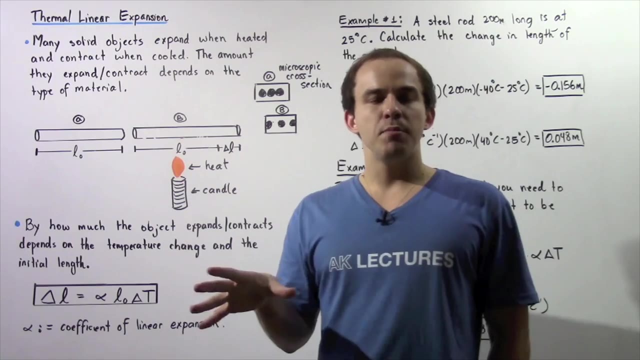 we're going to focus primarily on thermal linear expansion. So, as mentioned earlier, many solid objects either expand when heated or contract when cooled. So thermal linear expansion is a type of material that expands when cooled. The amount by which the solid object expands, or 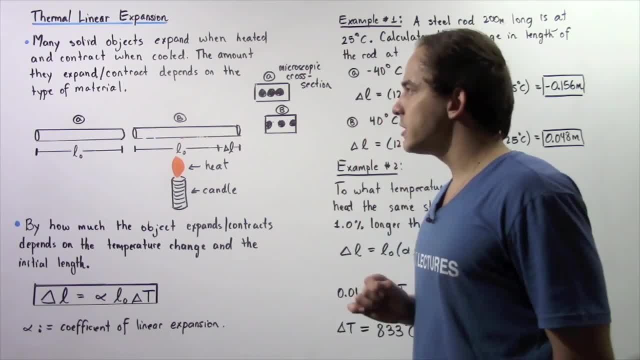 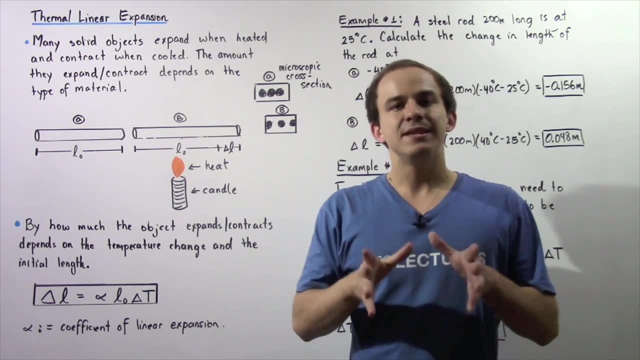 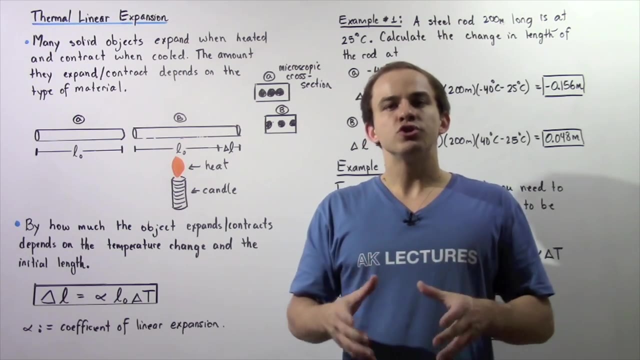 contracts depends on three things. Firstly, it depends on the type of material that the solid object is made of. In other words, it depends on the strength of the bonds between the atoms found within that solid object. So the stronger the bonds, the less likely our object will expand. 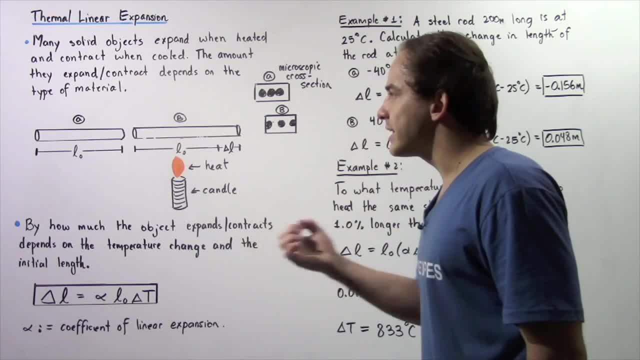 or contract. Now, by the way, thermal linear expansion is a type of material that expands or contracts or contracts along any horizontal axis. We'll talk about thermal linear expansion in the following video. Thermal linear expansion is a type of material that expands or contracts when heated or cooled. 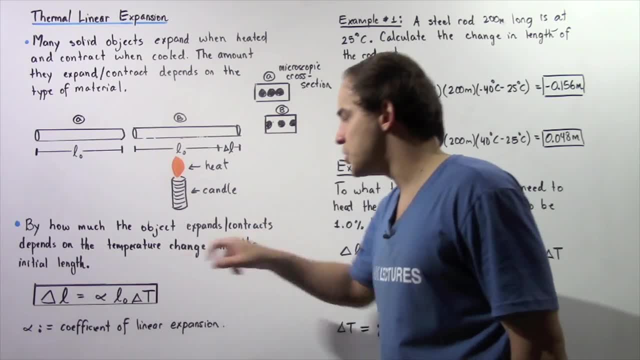 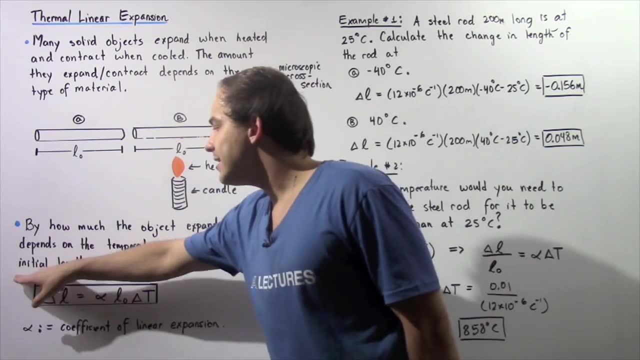 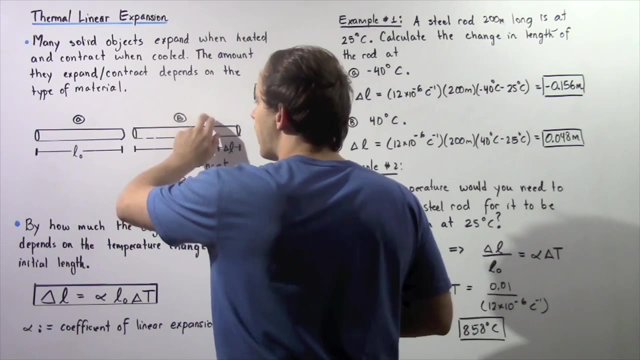 It also depends on two other factors: It depends on the temperature change that the solid object experiences and it also depends directly on the initial length of our object, of our solid object. So let's begin by looking at the following two diagrams: In diagram: A. we have our solid rod that has an initial length given by half. So for our solid rod, we have a solid rod that has a depth of 20 meters. On the other hand, we have a solid rod that has an initial length given by half. The length of the solid rod is 20 meters. as we 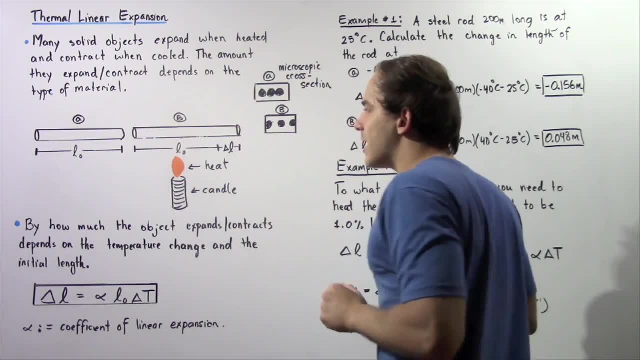 have to use the mass, the hundredth value. This is the difference between the two diagrams. In the previous video we learned that you can use the difference between the two diagrams and the given by L0.. And in diagram 2, we essentially take an energy source. so we take the following: 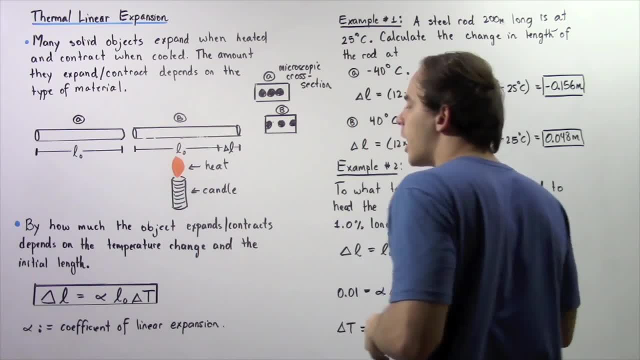 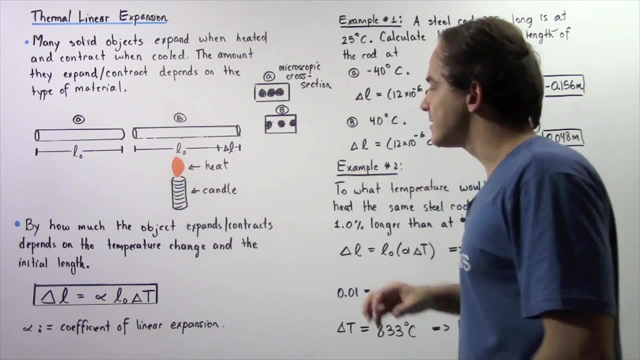 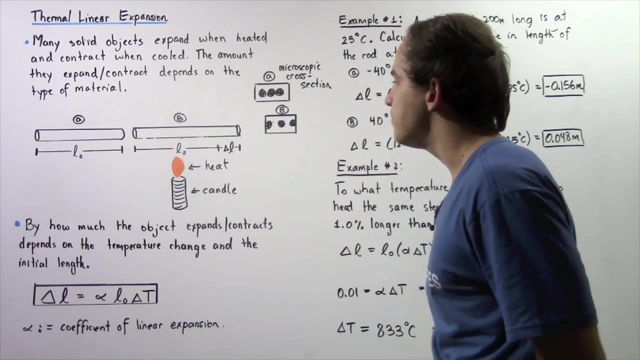 candle and we bring it very close to our solid object. So eventually that solid rod will expand outward along a linear axis, And the distance by which our rod expands is given by delta L, or simply change in L. Now what exactly is taking place on the microscopic? 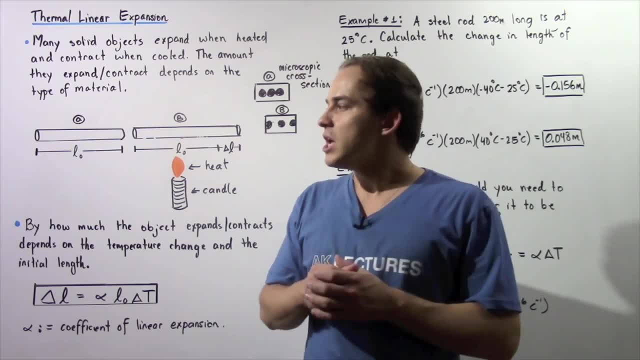 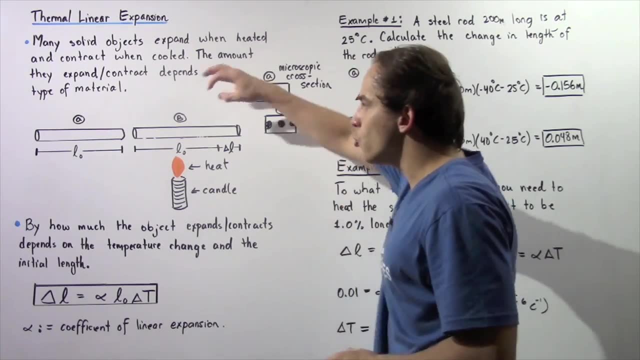 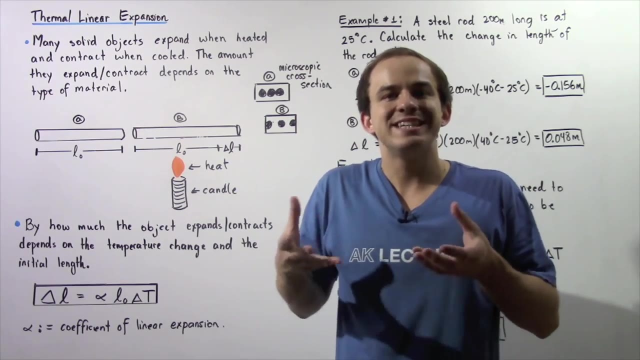 level to cause this expansion. So what's taking place is there's energy that is being transferred from this candle to the individual molecules found within the solid rod, And these individual molecules gain energy and they vibrate more violently, And so the distance between the 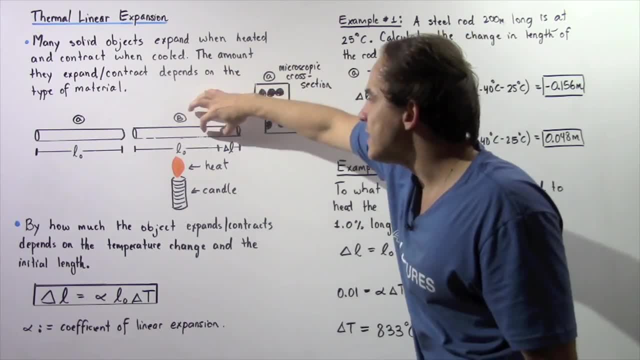 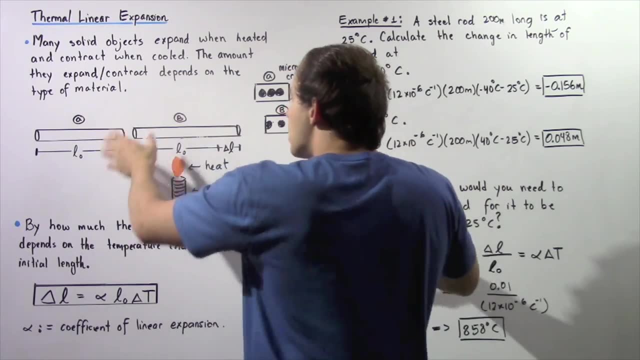 individual molecules and the solid rod is given by delta L, or simply change in L, And so the distance between any two adjacent atoms here is greater than the distance here, And collectively this increase in distance increases the entire length of the rod by an amount delta L. Now 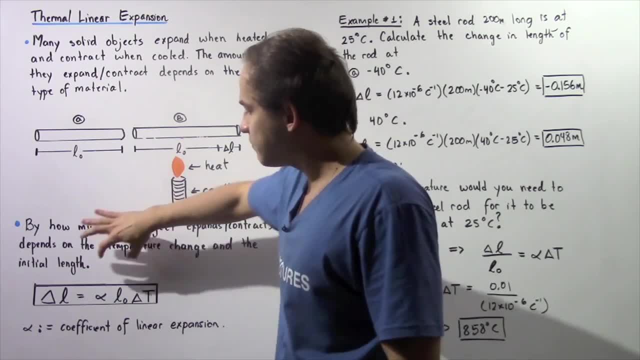 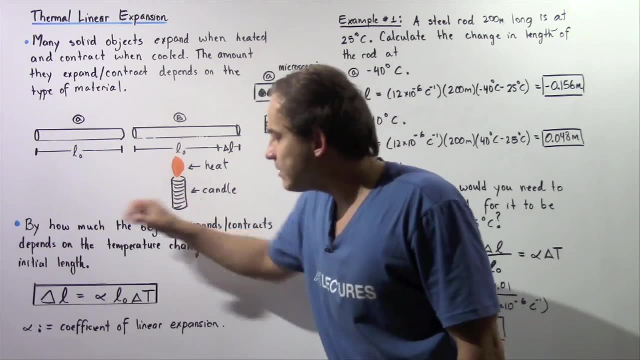 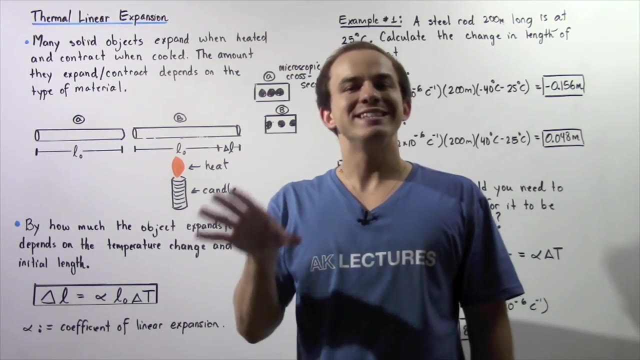 the actual formula that gives us the delta L is given by this equation. So the change in length of our solid rod is equal to the product of these three quantities. So delta T is simply the change in temperature given in Celsius. The L0 is simply the initial. 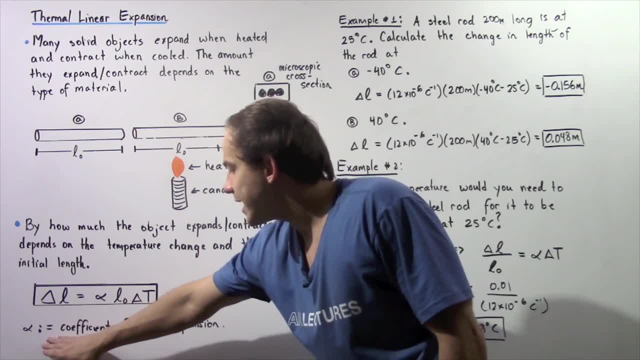 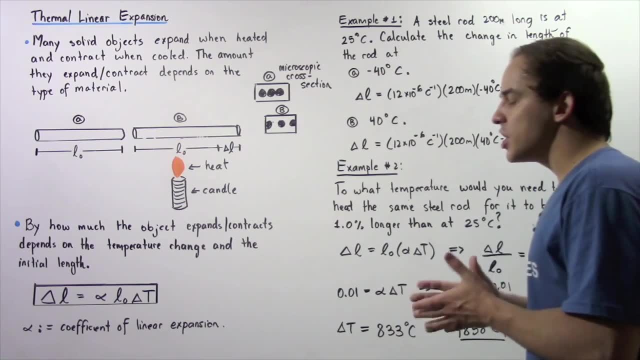 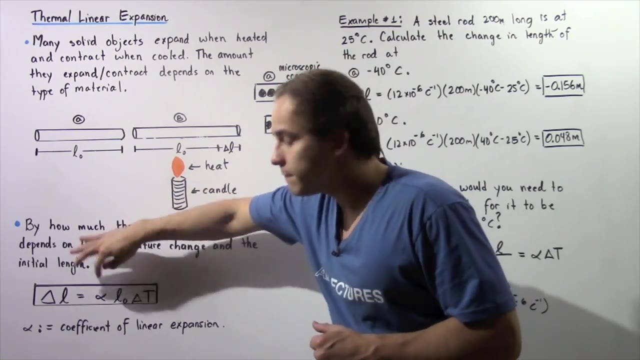 length of the rod, And our alpha is known as the coefficient of linear expansion. It depends on the type of solid that we are using. For example, steel rods and copper rods have different values of delta. Now notice the lower value of delta T. So the lower value of delta T is: 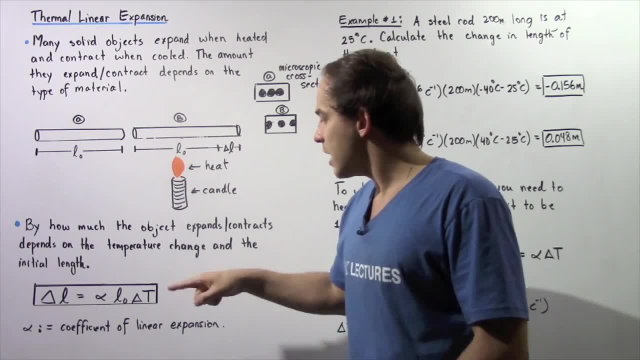 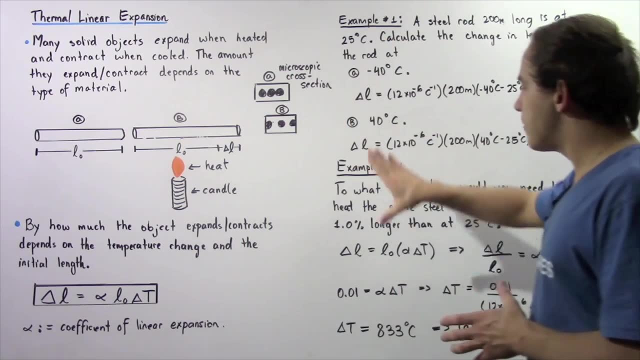 the constant value of delta T. So the higher the value of delta T is, the higher the value of delta T. So the longer our rod is, the more it expands, And the greater the change in temperature is, the greater that rod expands. So let's examine the following two examples. 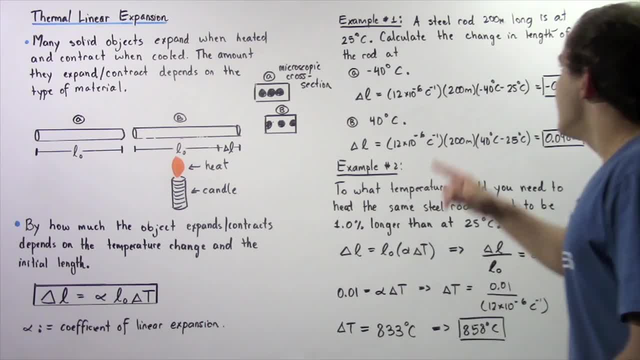 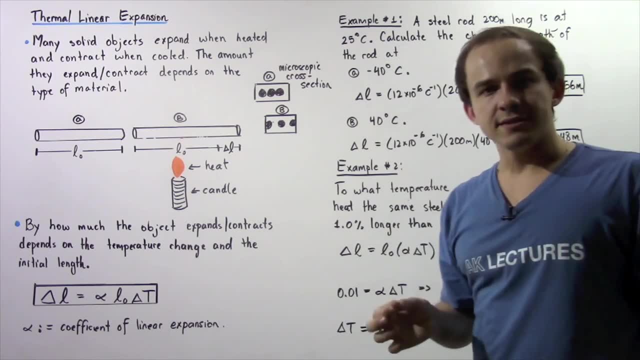 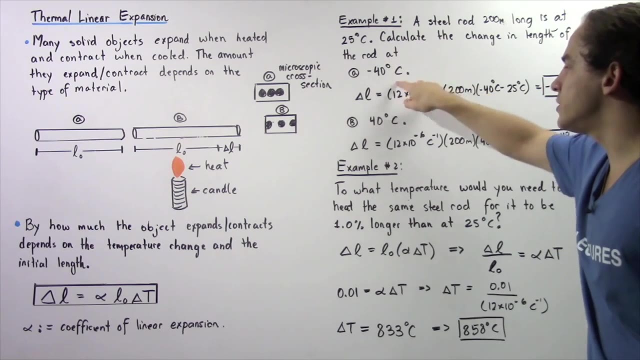 in which we're going to apply this equation. Let's suppose that a steel rod 200 meters long is at 25 degrees Celsius. Knowing that information, calculate the change in length of the rod at negative 40 degrees Celsius, And the change in length of the rod is at 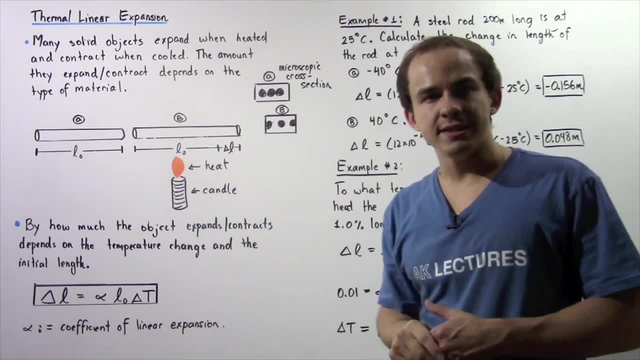 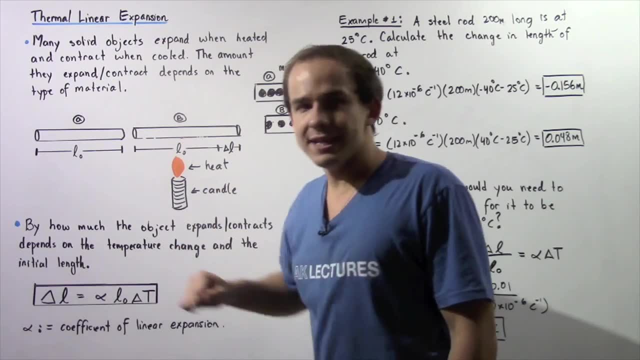 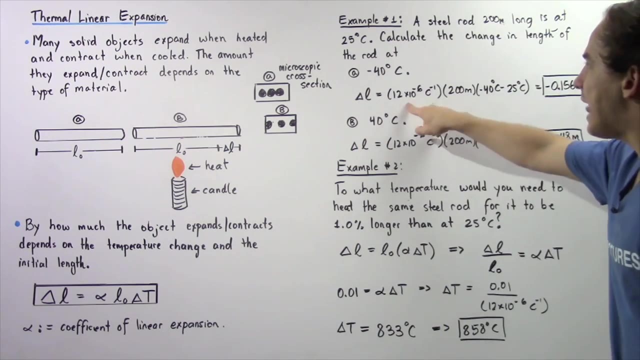 20 degrees Celsius And b at 40 degrees Celsius. So we essentially have to use this equation, So we have to determine what the alpha is for steel. So we can find the alpha in a textbook or online And we see that the alpha for steel the coefficient of linear expansion of steel. 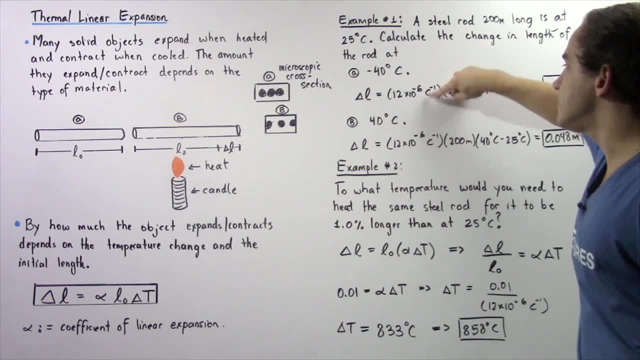 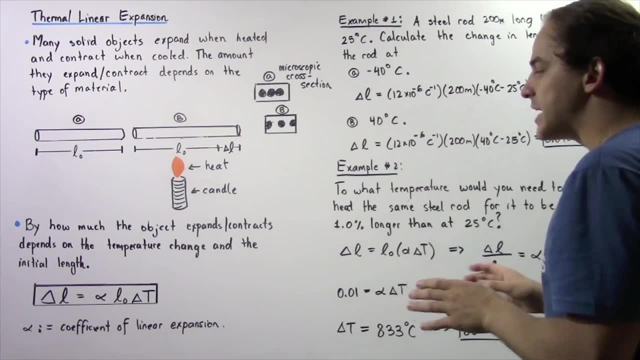 is 12 times 10 to the negative, 6 Celsius to the negative 1.. So we take this, we make it one dash with the 1 on the core, we'regrouping these two together, But now we have some global temperatures of about 10 degrees Celsius. Now you already have an answer. Again, we 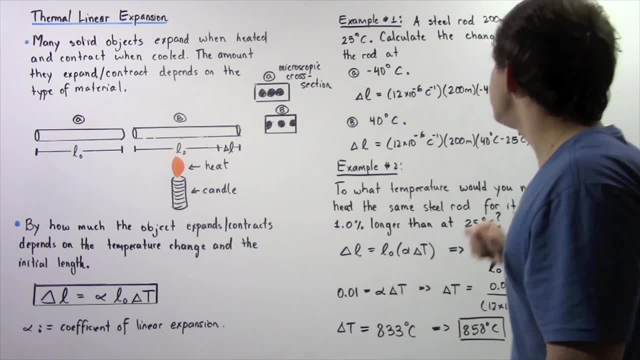 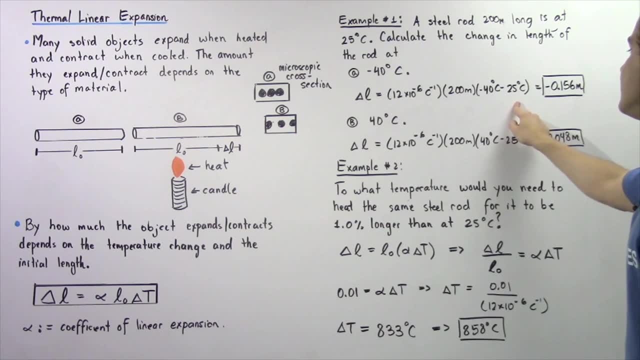 are not including 56 degrees Celsius here, So we just have to do some calculations and the final value of temperature is equal to 25 degrees Celsius. We add just the number of degrees in this table, and that equals negative 11 degrees Celsius. So what? Oh, so we have. 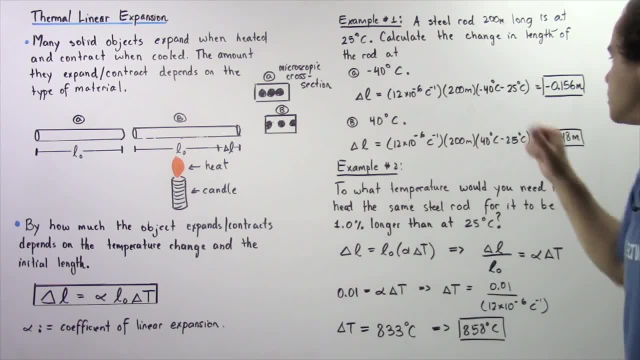 35 degrees Celsius. here we smooth out. But because at könnt temp temperature is correct, we just remove the image from here. But unlike other variables, we require the temperature negative 0.156 meters. So this negative simply implies that our solid rod contracts and not 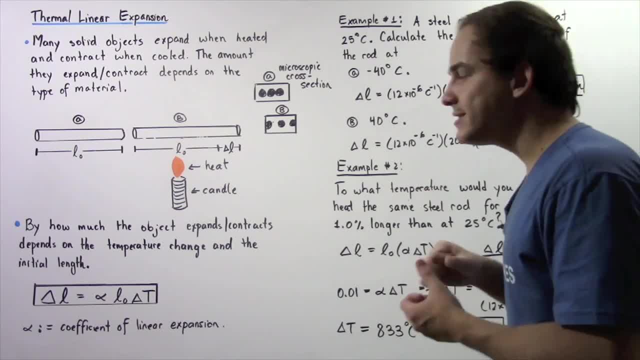 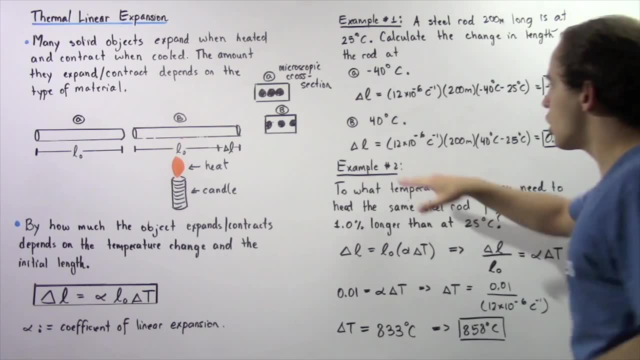 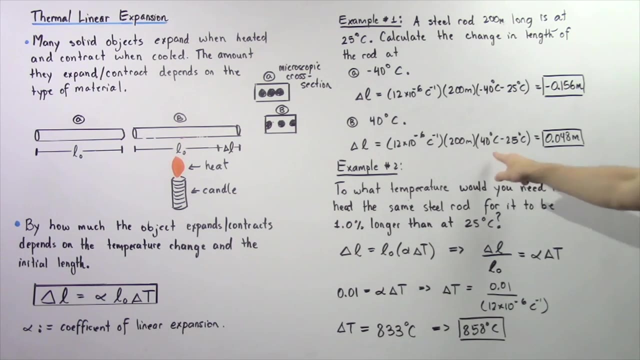 expands, It contracts because the temperature decreases, So the molecules vibrate less violently and the distance therefore decreases. So let's move on to part B, 40 degrees Celsius. So we apply the same exact formula, except now the final temperature is 40 degrees Celsius. 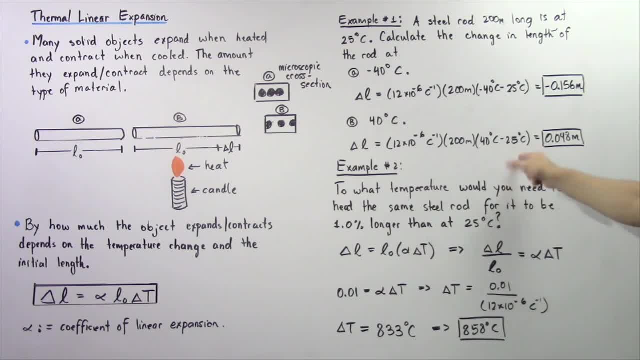 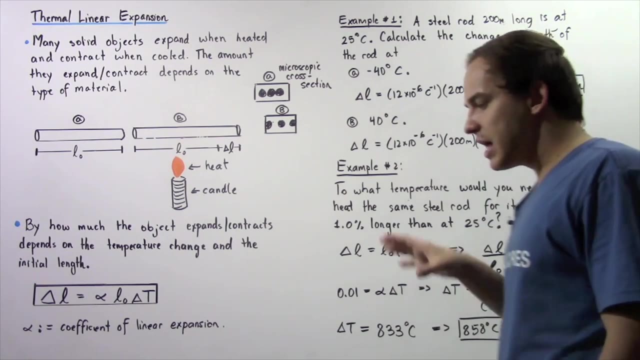 So we have 40 degrees Celsius minus 25 degrees Celsius gives us a change in temperature of 15 degrees Celsius. 15 times, 200 times this quantity gives us positive 0.048 meters. So the positive simply means that our solid rod expands because there is an increase in. 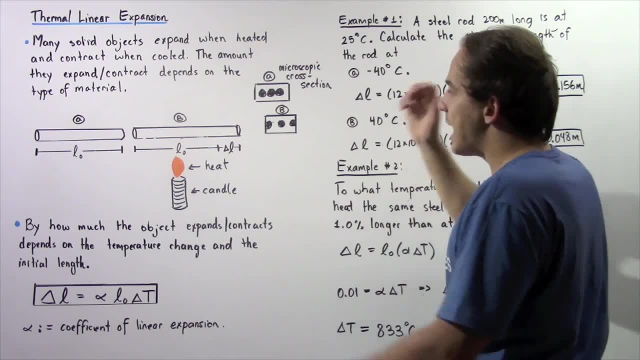 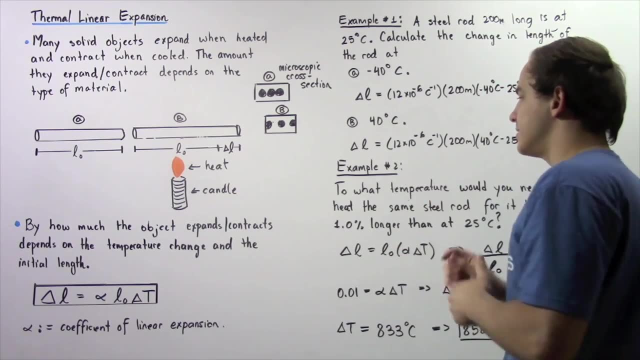 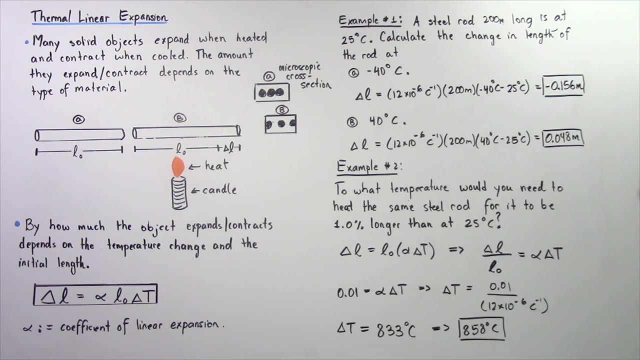 temperature and the microscopic atoms and molecules vibrate more violently, and so the distance between any two adjacent atoms increases. Now let's examine example two. To what temperature would you need to heat the same steel rod as in example one for it to be increased by one percent? So you want to